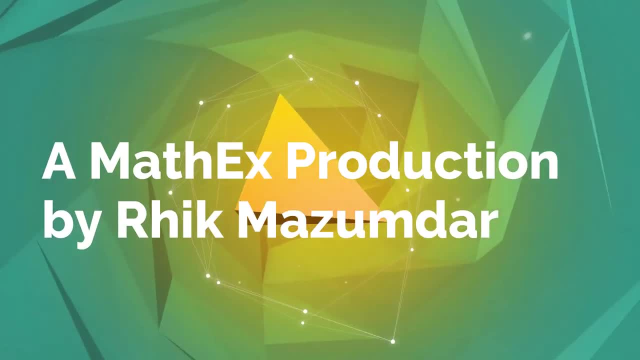 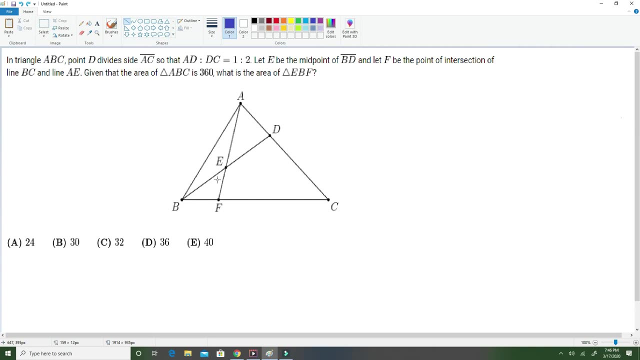 Hello, today we'll be going over number 24 of the 2019 AMC-8.. This problem in particular is quite interesting because, even though it's an AMC-8 problem, it looks a lot like an AMC-10 problem In future years. it wouldn't surprise me if this comes up as number 13 or 14 on the AMC-10,. 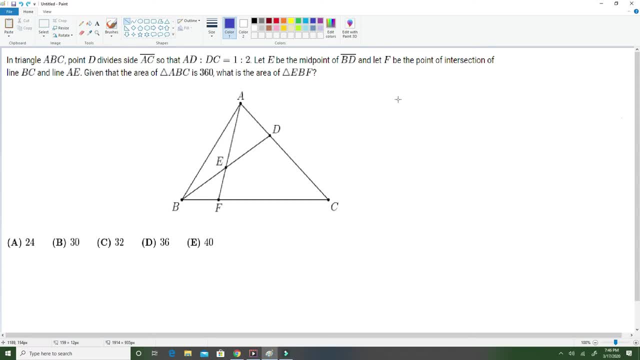 as this level of geometry is not really common in the AMC-8 test, Without further ado, let's get to it In triangle ABC. point D divides sides AC, so that AD and DC equals a 1 to 2 ratio. Let E be the midpoint of BD and let F be the point of intersection of BC and AE. Given that, 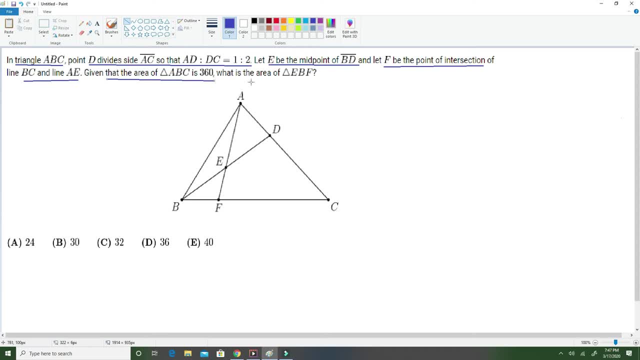 the area of triangle ABC is 360,. what is the area of EBF? Right now, we're trying to find the area of triangle EBF. We don't really know anything about it, so let's label it as X. What do we know? We know that the area of triangle ABC is 360, and that will be probably. 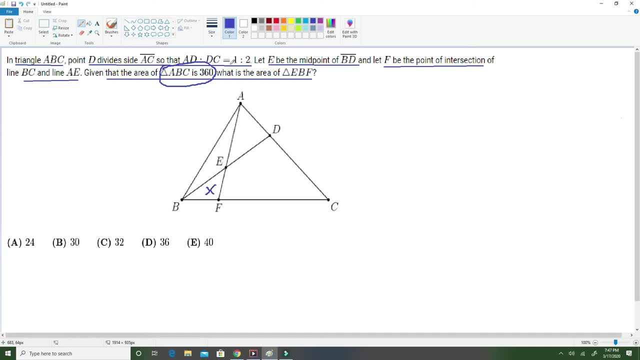 crucial into finding the area of EBF, as the only other information we got is the 1 to 2 ratio between AD to DC. If AD and DC are in a 1 to 2 ratio, that means if we label AD as A in this. 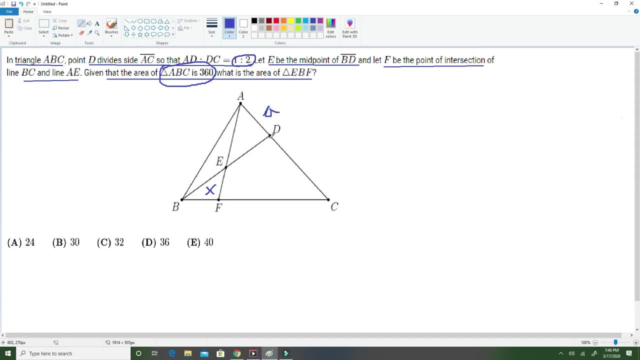 case, because we already have X there. If AD is A, that means DC must be 2A. One thing we can notice by looking at this triangle itself is that triangle ADB and triangle CDB both share the same height but different bases, and we know the ratio that. 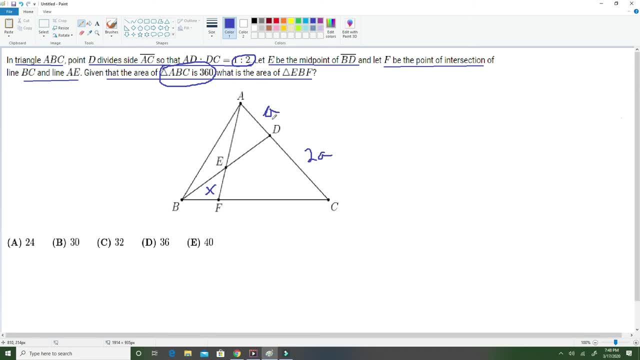 their bases are in with one another. This can correlate to their area: The area of triangle- CDB- is the same height but different bases. This can correlate to their area. The area of triangle- CDB- is the same height but different bases. This can correlate to their area: The area of triangle. 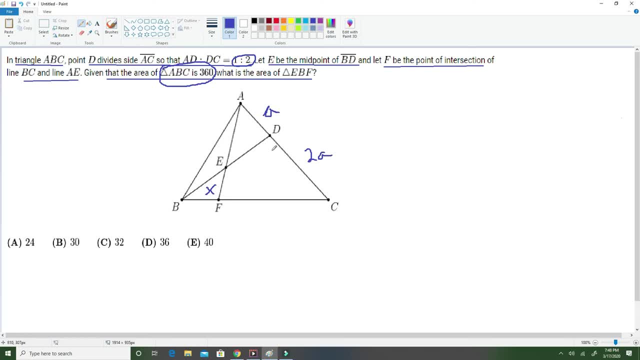 CBD is also twice the area of triangle ABD. Using this information, and that they sum up to 360, we can determine that the area of triangle ABD is 120, while the area of triangle BCD is 240.. Going one step further with this, we can also see that the same thing. 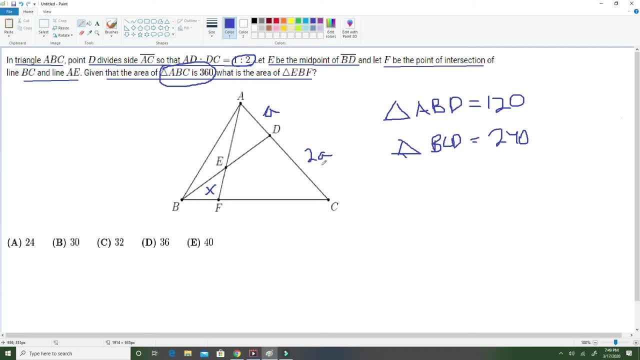 we observed with the triangles ABD and BCD can also be observed with the triangles ABE and AED. Both these triangles share the same height. If they share the same base and the same height, the area of the triangle is the same. The area of the triangle BCD is the same base. 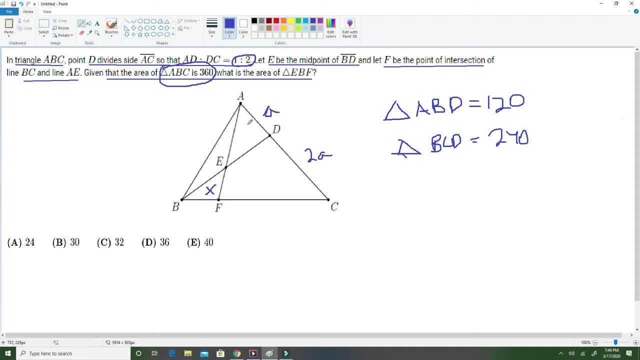 times height over two. so, considering all these factors are the same, we can say that the triangles ABD and AED have the same area. Since they have the same area and both their areas combined equals ABD, which we know is 120, we can say that the triangles ABD and 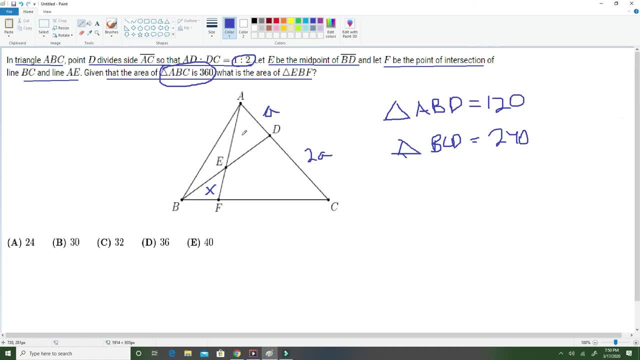 and AED each have an area of 60, which you can draw directly into the diagram. From there, we notice that we have this huge quadrilateral region that we don't know anything about. In order to make this easier to deal with, we could probably turn it to a couple triangles, as it's easier to find the area of a. 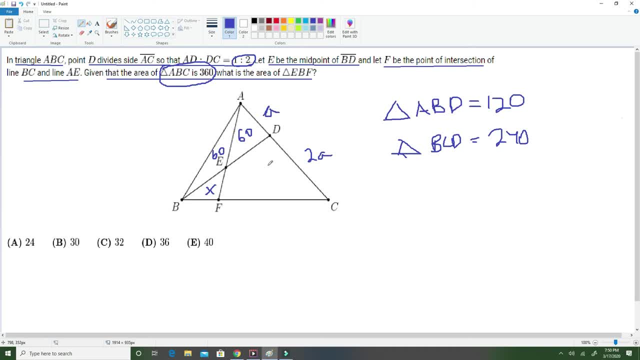 triangle than it is than this irregular quadrilateral. So we draw auxiliary line EC. Then we notice the similar relationship that we've seen several times throughout this problem: Two triangles with the same height but bases that are in the same proportion to one another. In this case we notice that 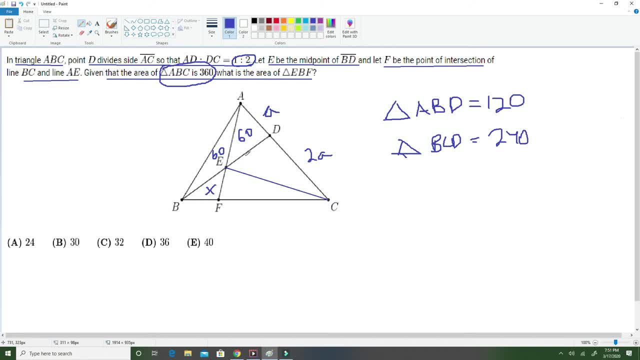 triangles AED and triangles EDC have the same height, but just like triangles ABD and BDC, one of the bases is twice the others. This means that the triangle ABDC is the same height as ABDC. This means that the triangle ABDC is the same height as ABDC. 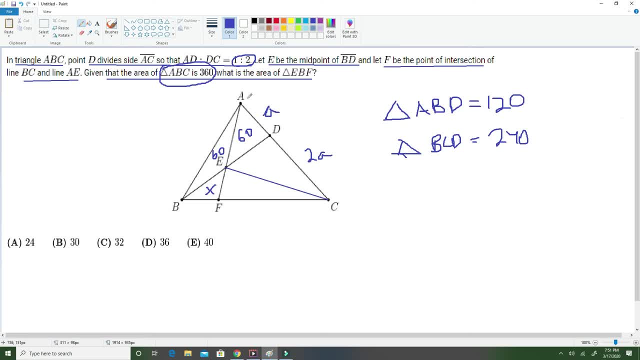 This means that the triangle ABDC is the same height as ABDC, that one of the areas is exactly twice the others, Since we know that triangle AED is equal to 60,. we know that the area of triangle ECD is 120, because it's supposed to be exactly twice the. 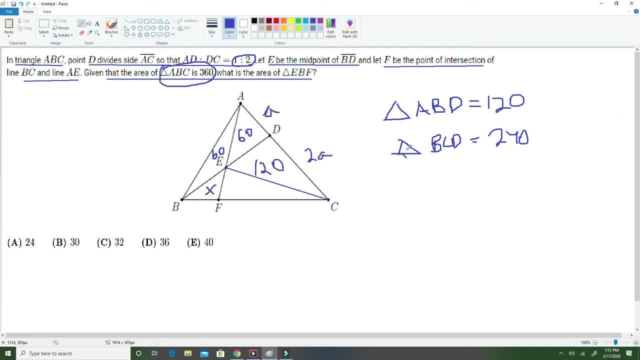 area because their bases are twice as much. So then we write in: area of triangle, EDC is 120.. That leaves us with one final area in our triangle. The area of the triangle, as it tells us, the problem is 360.. So far, adding up all the areas, we get the areas of our known parts to be. 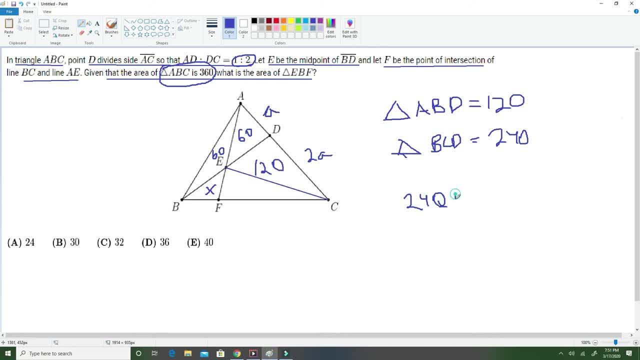 240 plus x, with our unknown part being the area of triangle EFC. In order for it to be 360, whatever EFC has to equal has to be 360. And after subtracting 240 plus x from both sides, we see that triangle EFC must be equal to 120. 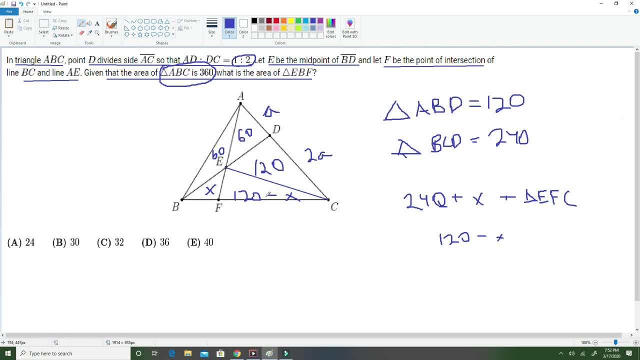 minus x. So now that we know all these areas, we can kind of do what the reverse we did to get said areas, To get these areas, we compared the bases and created areas based off those. But now, using these areas, we can use the, we can create relationships between the bases. So let's look at line 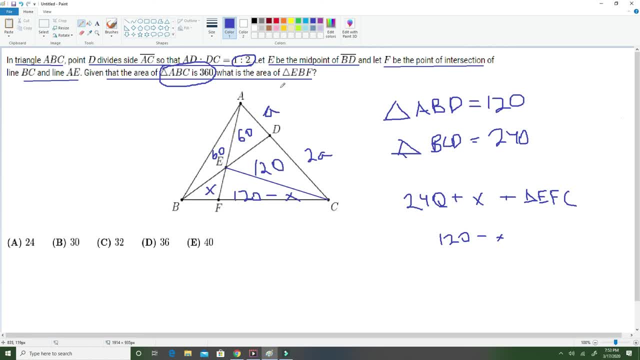 let's look at the area of x, because, anyways, that's what we're trying to solve in the grand scheme of things, because x represents the area of our unknown region, EBF. So there's several lines we could hunt for in terms of x, But it seems that EF. 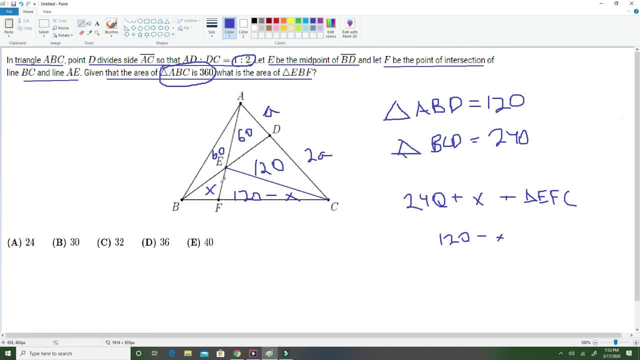 is probably the best line to compare, And since EF is on the same line as AE, it seems like it's a, it's a good idea to compare these two with one another. So then, if we set up the relationship between EF and AE, what can we say? Well, we see that triangle- BEF and BEA- both share these lines. 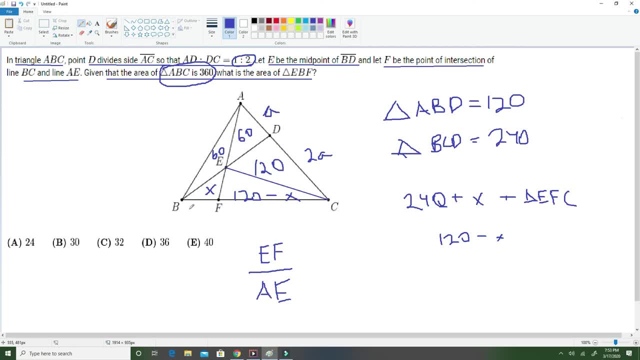 as bases, but they also share the same height. So whatever the ratio between the bases are, it also is the relationship between between the areas. So since we said that relationship between the bases EF and AE is EF over AE since they share the same height. 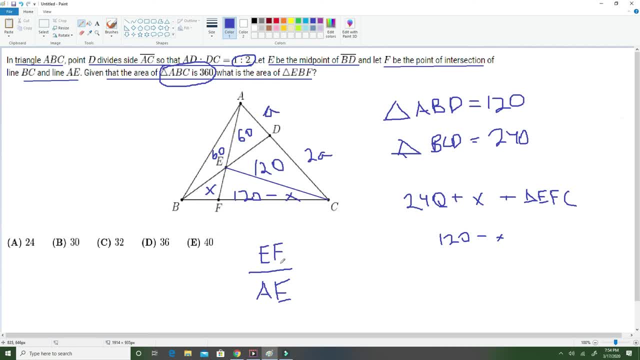 we can also say that the areas are also in the same relationship. So we get that EF over AE is equal to x over 60.. Now if we flip over to the other side of AE and EF, we can see the similar kind of thing happening on the other side: Triangles ACE and triangles ECF. both have the 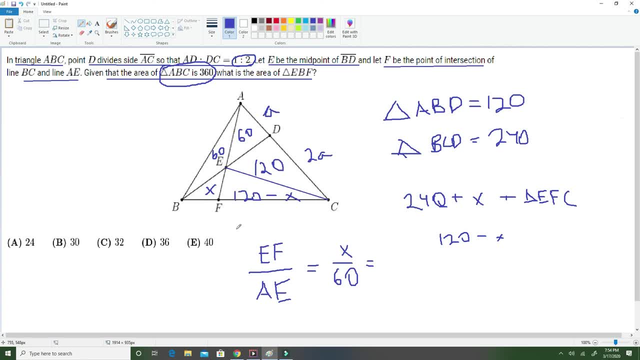 same area. So we can write their areas in the same kind of way. We are going to write: 120 minus x over 180 is equal to EF over AE, which is equal to x over 60. With that we get a relationship in terms of x which we can solve in order to find the value. 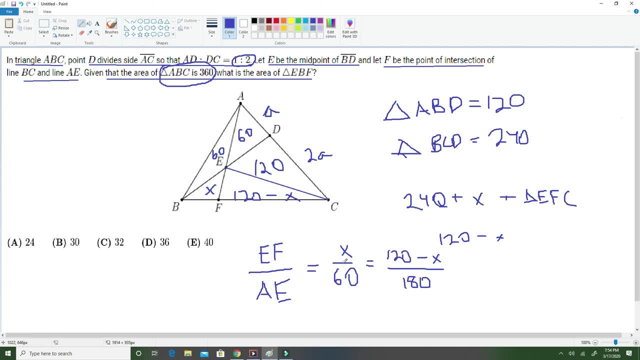 of x and thus find the area of EBS Great. thank you again for choosing this subject. Thank you for spending your time with us this talk. If you have any questions, let us know in theال on our website. We're always happy to succeed in sharing our baluts. 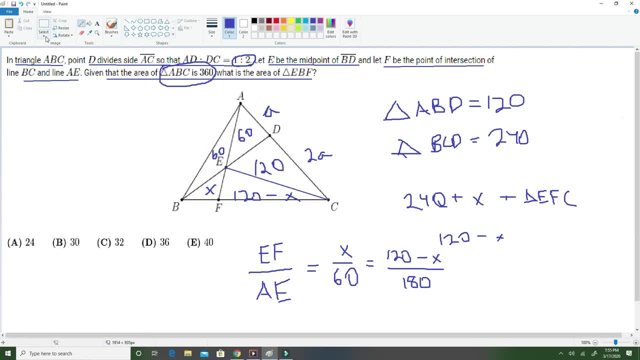 See you in the next one. find the area of EBF. So if we cross, multiply these two parts, we get 180x is equal to 7200 minus 60x. Then if we bring all the x's to the same side, we get 240x. 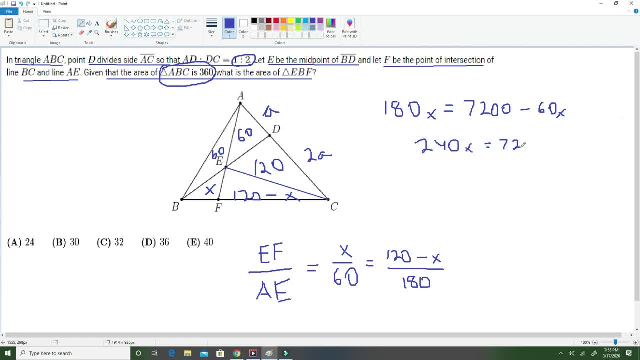 is equal to 7200.. Divide by 240 on both sides, we get x is equal to 30. And, as I've said earlier, x is the area of EBF. So, since we know the area of EBF is 30, that is the right answer. Thus, the answer is B. 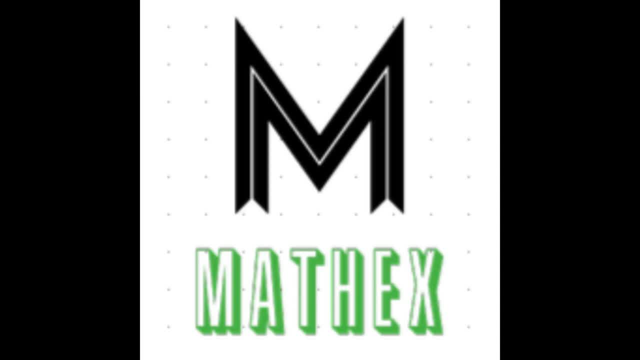 Thank you very much for watching.